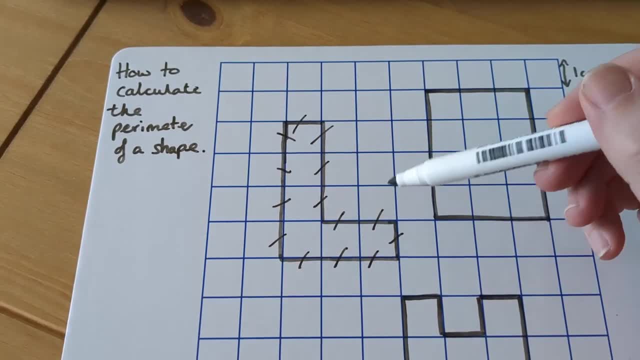 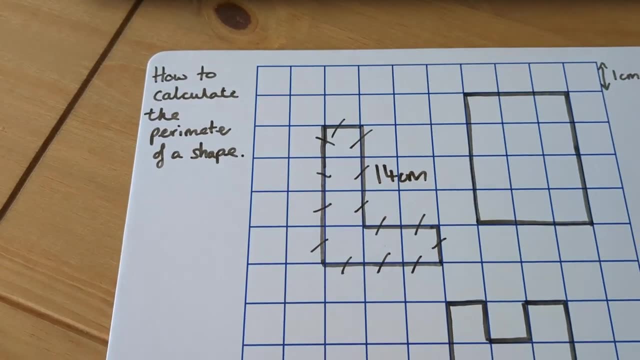 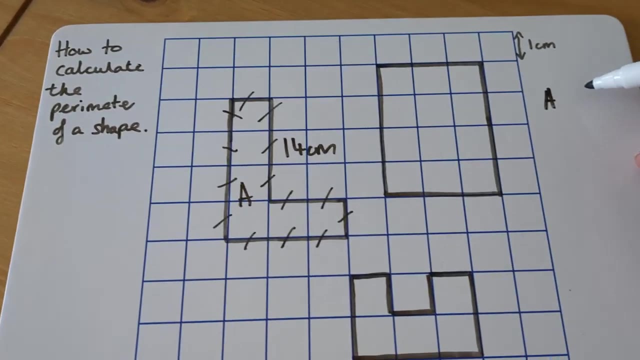 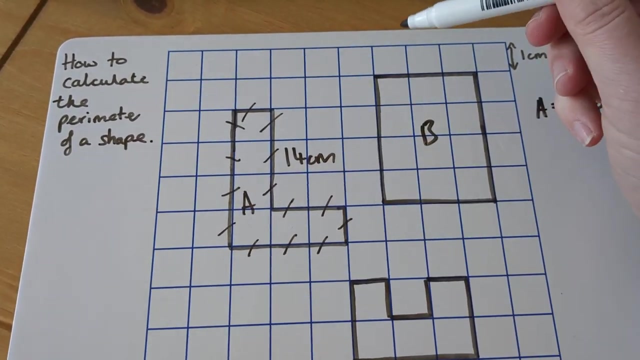 So in total there are 14 sides here, each one a centimetre. so we can say that that is the perimeter, The perimeter of this shape. let's give that a letter. we'll call that A. So A equals 14 centimetres for the perimeter. We'll do B and go around again. so 1,, 2,. 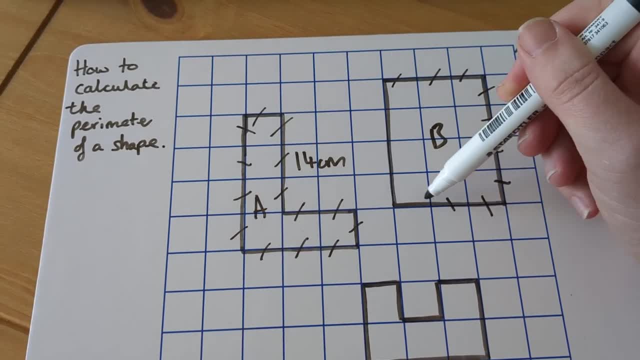 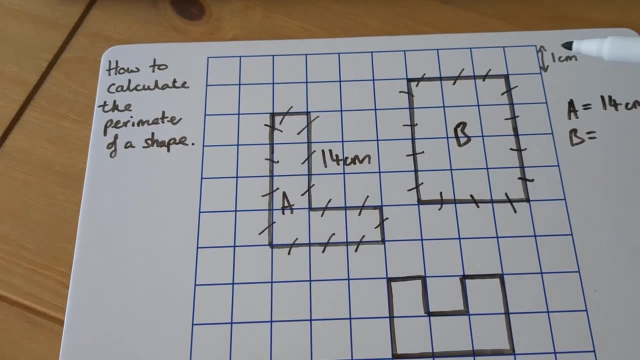 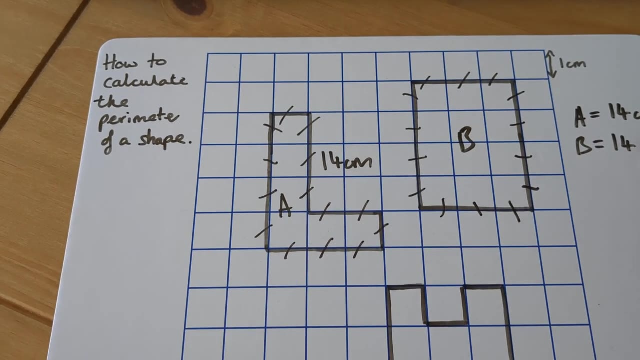 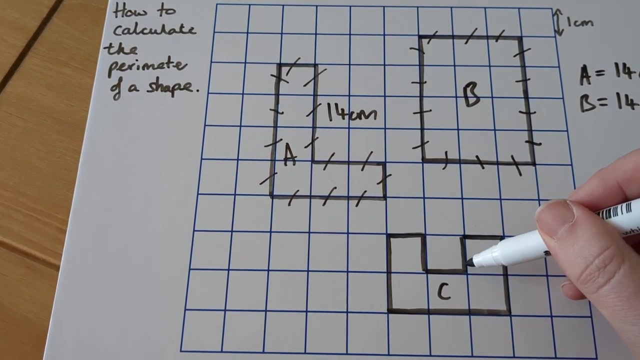 3,, 4,, 5,, 6,, 7,, 8,, 9,, 10,, 11,, 12,, 13,, 14.. So B: the perimeter is awful on what it was: 11,, 12,, 13,, 14,- exactly the same Funny coincidence. And C: we can start anywhere, but don't forget. 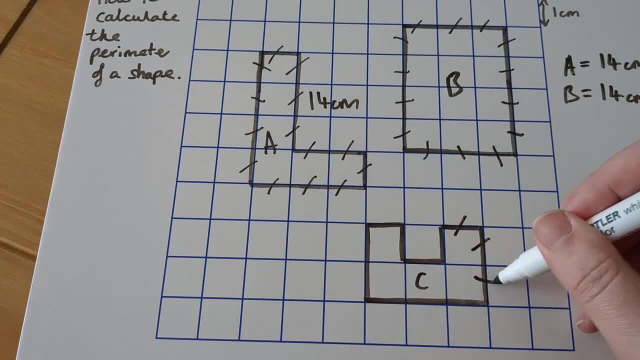 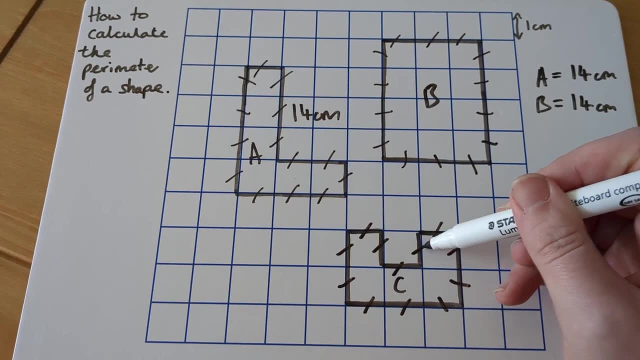 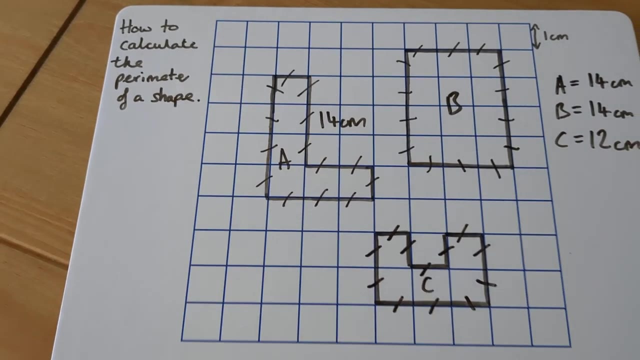 that this one goes inside as well. So we've got 1,, 2,, 3,, 4,, 5,, 6,, 7,, 8,, 9,, 10,, 11, don't forget that one- 12.. So this time C, the perimeter is 12 centimetres And that is a. 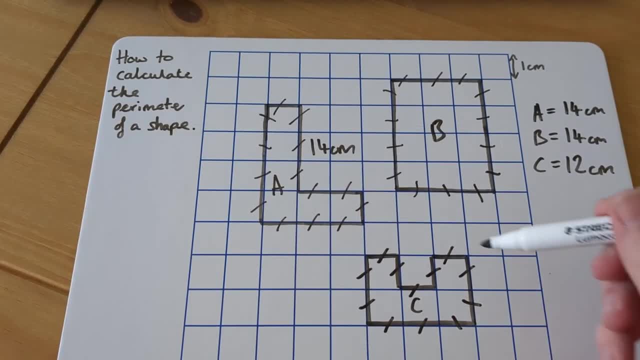 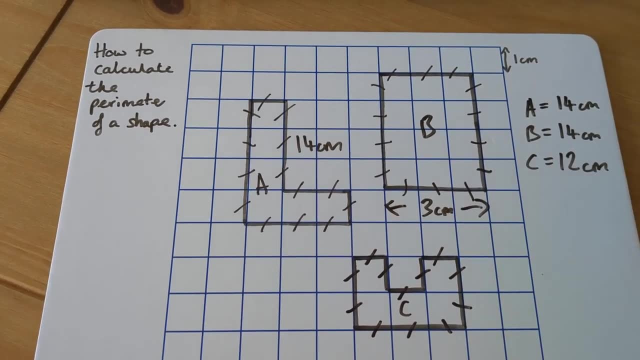 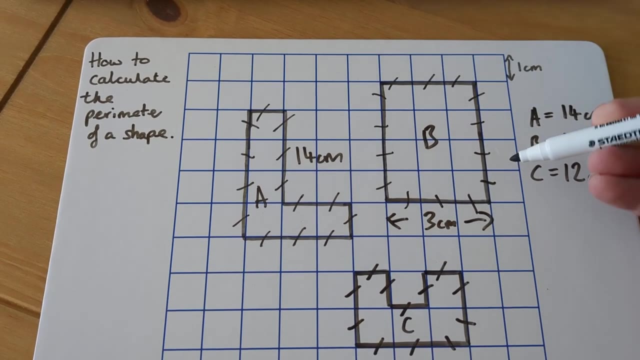 really easy one. It's a really easy way of doing perimeter. Eventually we'll have labels on this, so I'd say things like this bit here is 3 centimetres, so we won't need to count all the squares because they won't be there, But if we know, this is 3 centimetres and up here is 4 centimetres. 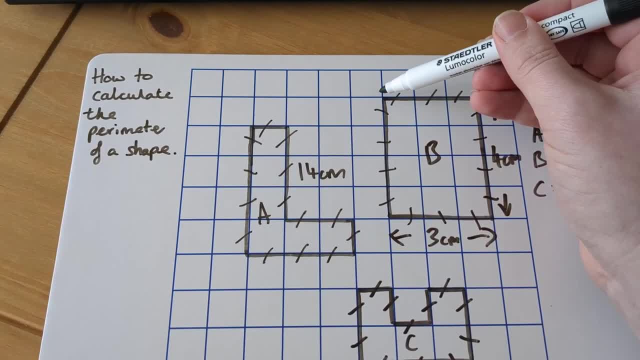 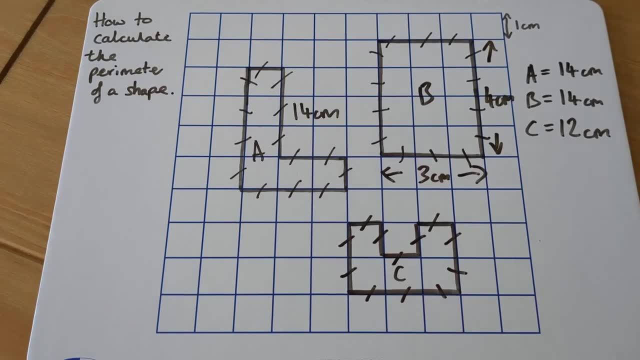 we can say: well, that's 3,, add 4,, add another 3, and add another 4.. And that's a different way of working out perimeter when you don't have the squares. But for today it's just squares. So this is the sheet that I have for you, So have 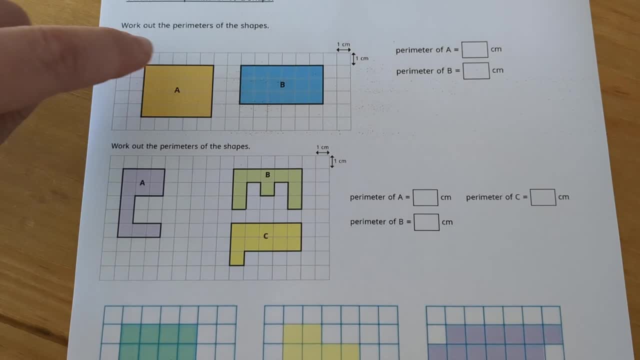 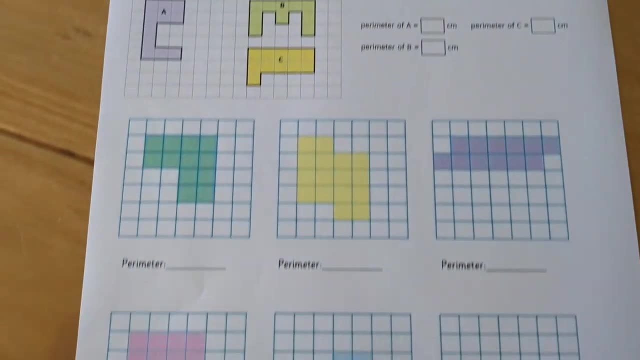 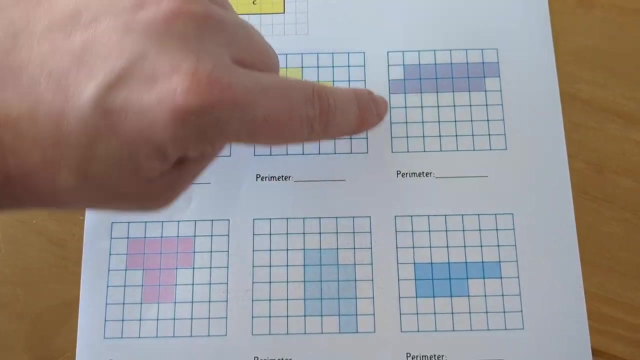 a go at this. Work your way around the perimeter, counting those squares to find out what the perimeter is for A and B. Work out A, B, C And then these ones, exactly the same. but don't be tricked by this. Even though it's right next to the edge, that is still a piece.